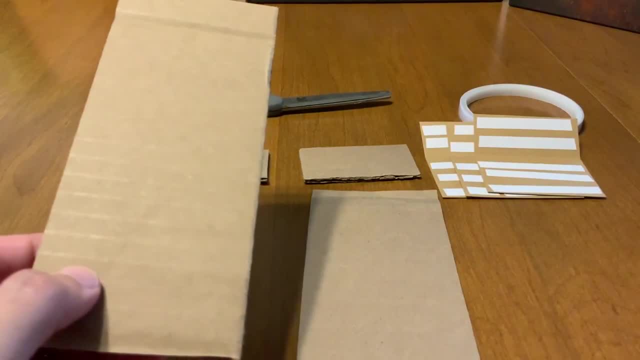 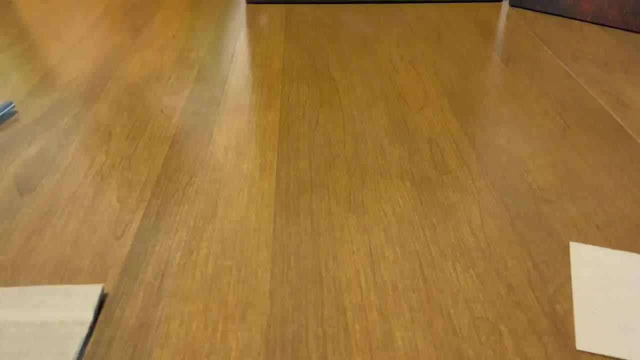 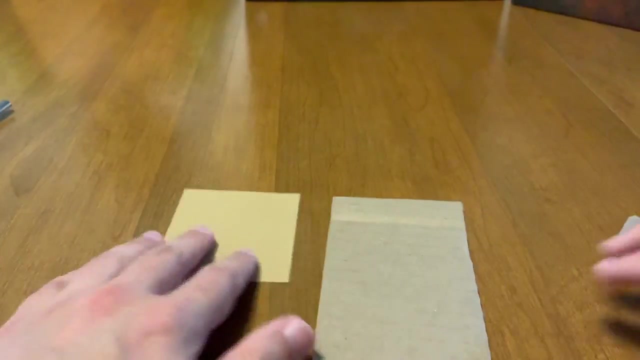 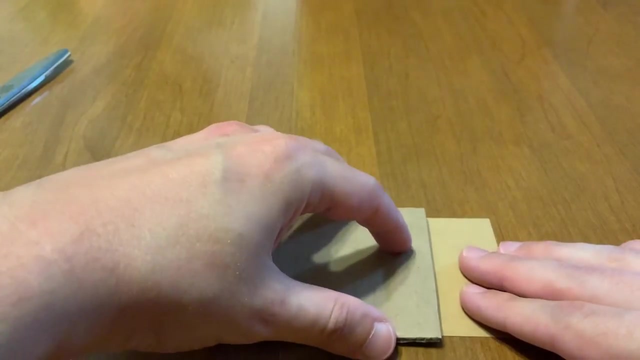 keep the corners together. So what I'm going to do: I'm going to grab and move this out of the way so you guys can have a clear view of how it's done. I'm going to grab our cardboard that I want to place. Let me lower this down. What I'm going to do. I'm going to go and put it over like this: 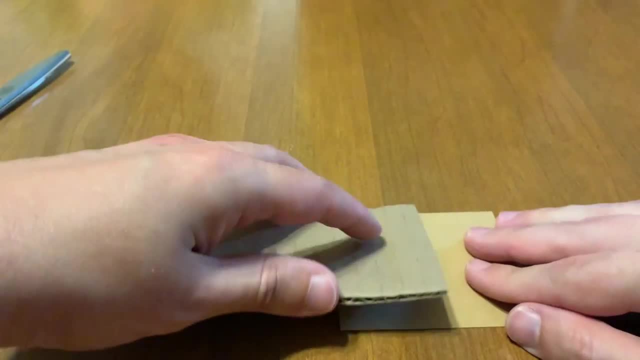 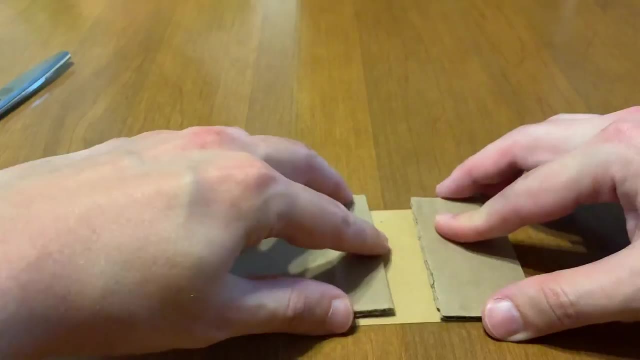 because I know that I want it to stick to the bottom of the box. So I'm going to go ahead and to the back right here. but I also don't want it to stick out. So I'm going to go and put this smaller piece in a way so it doesn't go, it doesn't stick out like that, but it covers it. 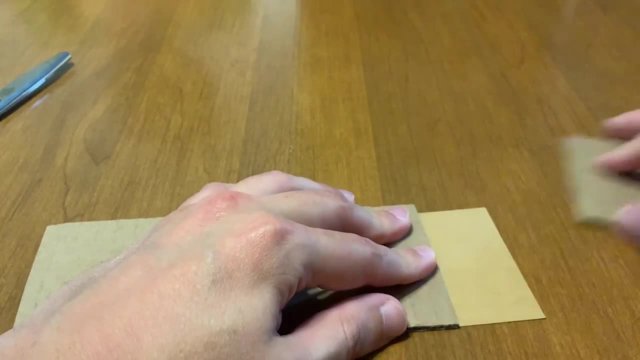 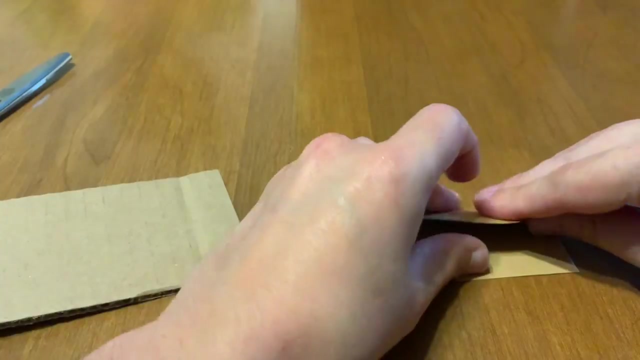 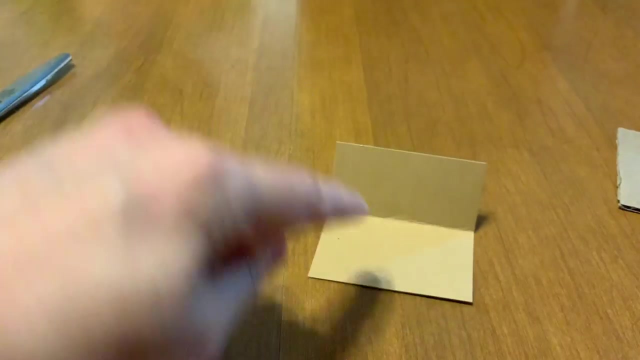 completely Okay. so now I know that's how big I need it. So what I do? I hold down this edge and I just lift up and finish the fold. So there I go, I have my edge That I'm going to use to tape the corners together. So then next, what I do? I grab double. 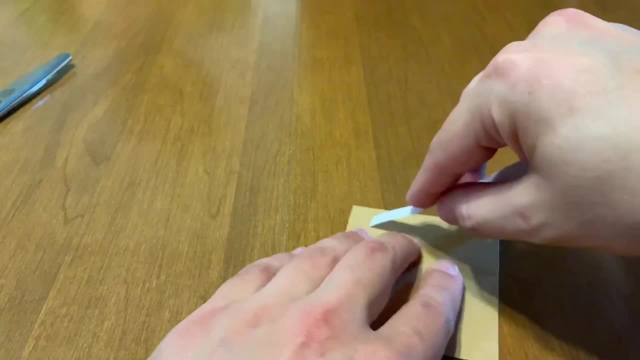 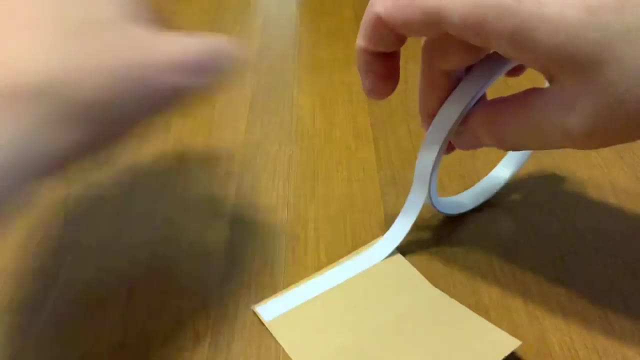 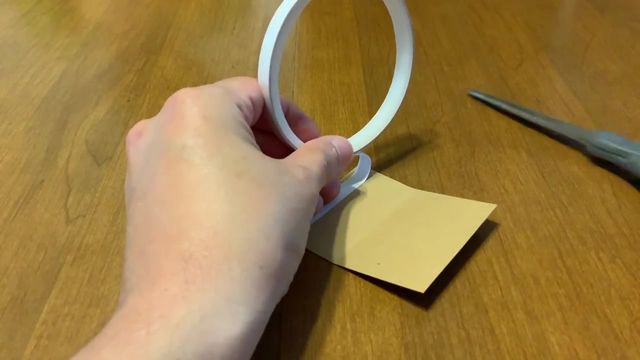 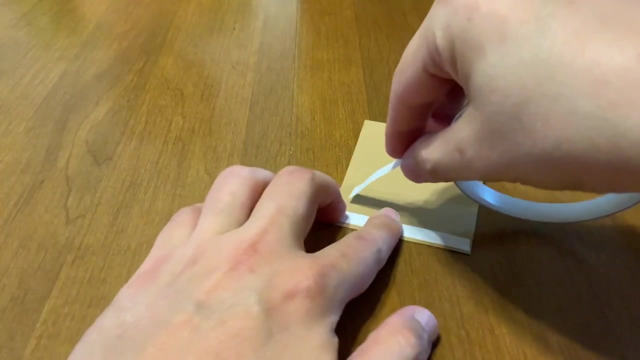 edge tape and what I do. I just carefully kind of manage my way around this corner. I should have the scissors closer to me, right, And I cut, right there, I go ahead and I do it one more time I like to do. I like to put it two or three times, depending on the size. 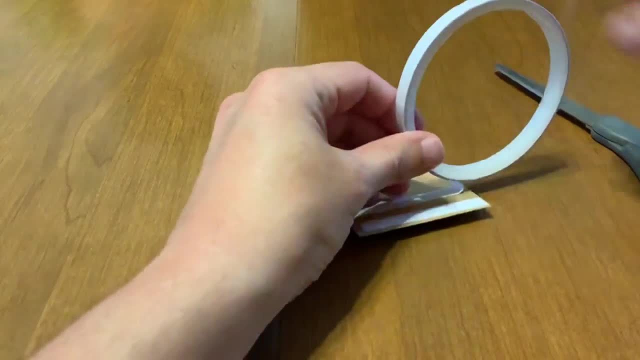 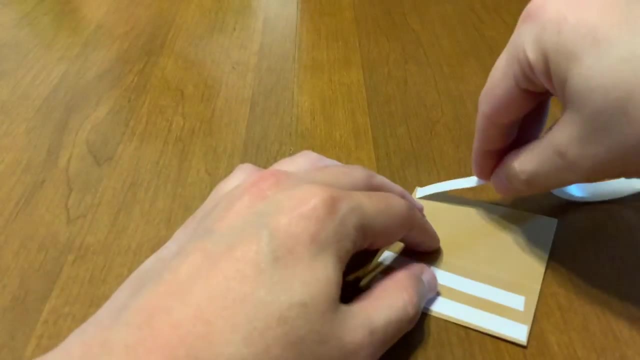 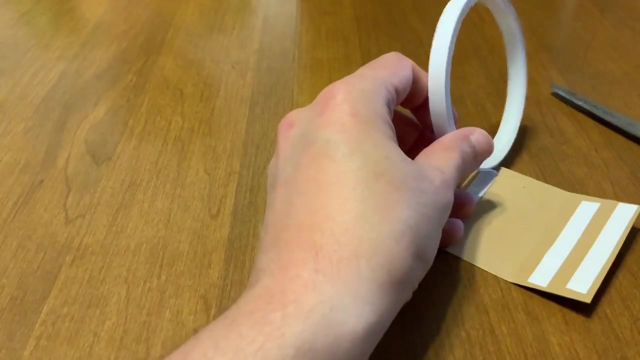 of the cardboard And then I go ahead and do the same thing on the other side. I hope you guys could see this clearly and my hand's not in the way too much. I just really need you guys to get an idea of how simple really it is to do this. 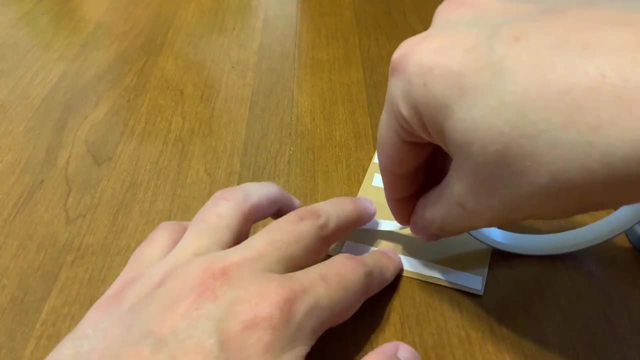 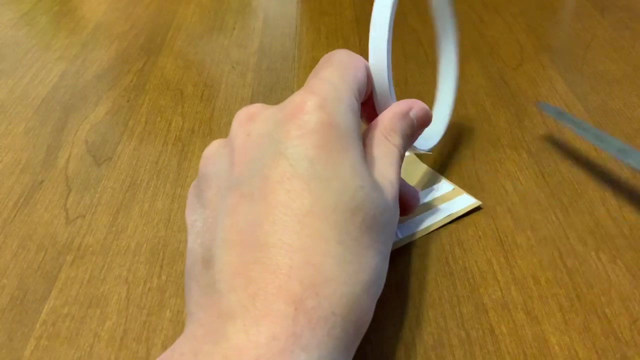 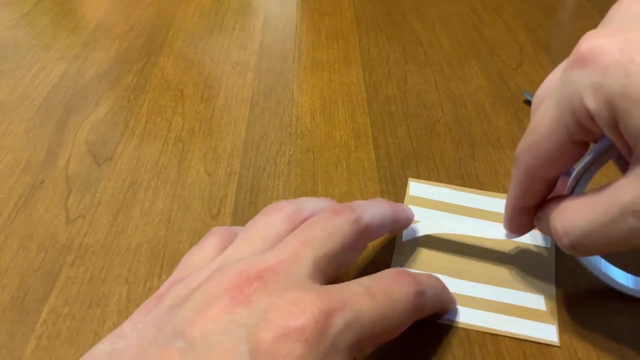 Because I personally was. I was intimidated when I was first thinking about it. I didn't think I could do it, And one day I ended up getting something shipped to me and I was like, hey, you know what? There's some cardboard there, Might as well try it. And since my wife does a lot of crafts work, 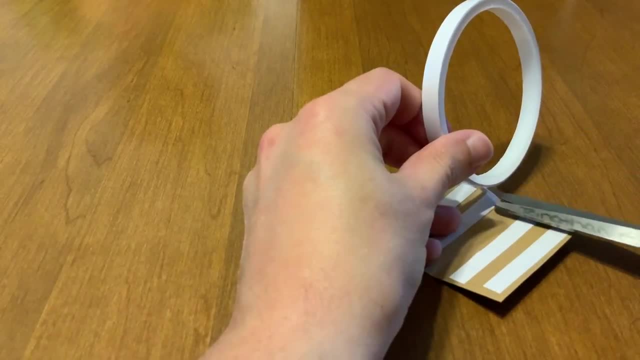 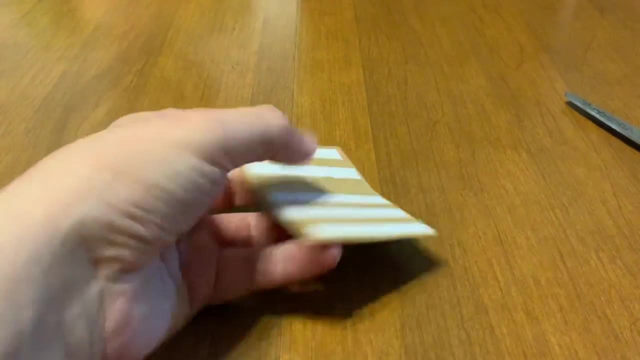 with Cricut and whatnot. I was like, hey, you know what, I'm going to use some of her material and try to create my own inserts. So there you go. That's how I do the edges. So I'm. 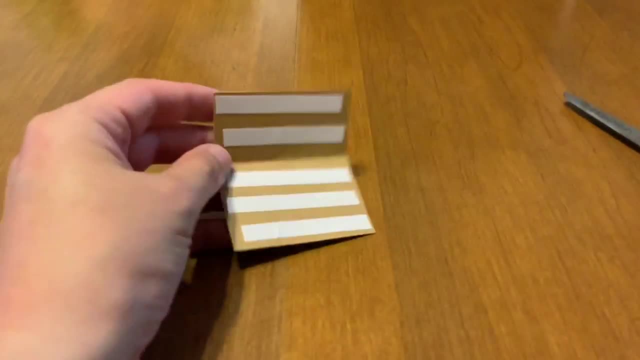 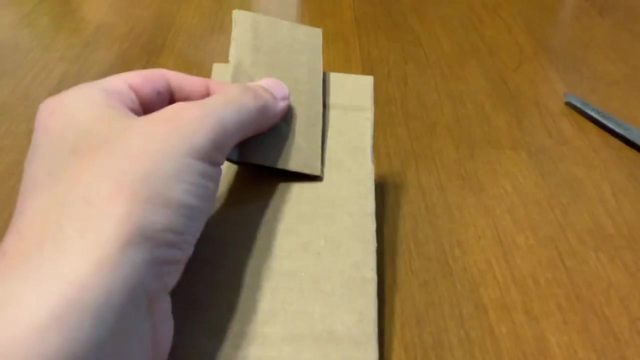 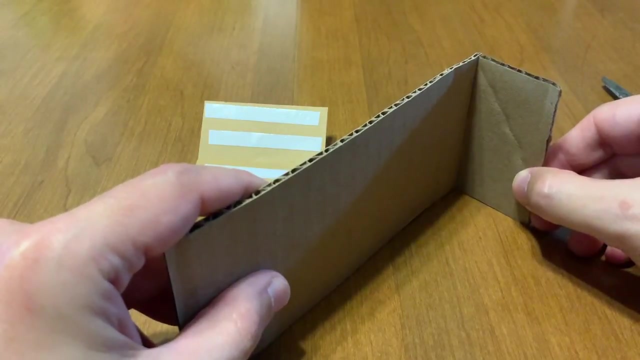 ready to start connecting the pieces together. So, basically, here I go. Let me make sure I get the one that goes with it. Okay, here we go. These are the two pieces, and the idea is that I want to put the pieces together like this, so it 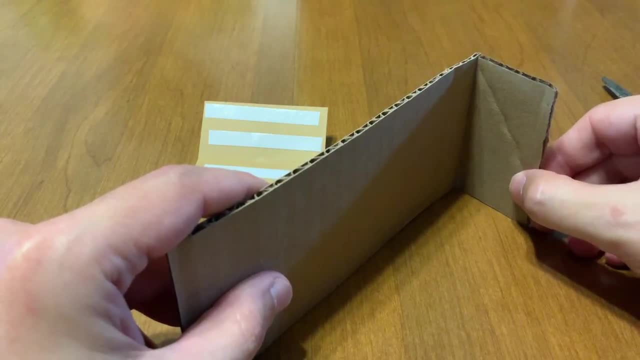 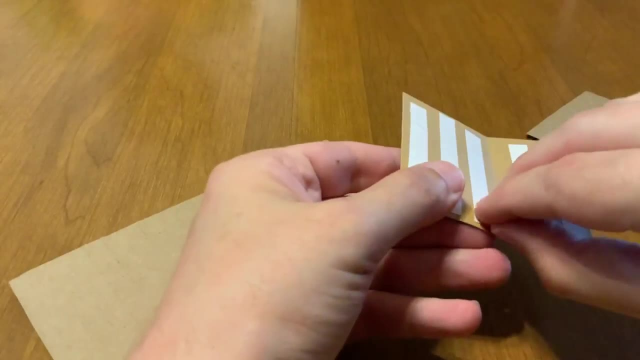 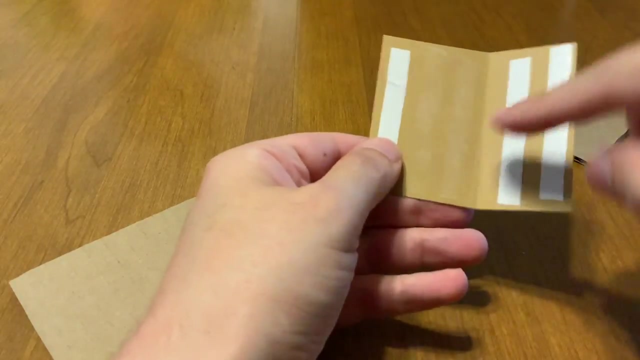 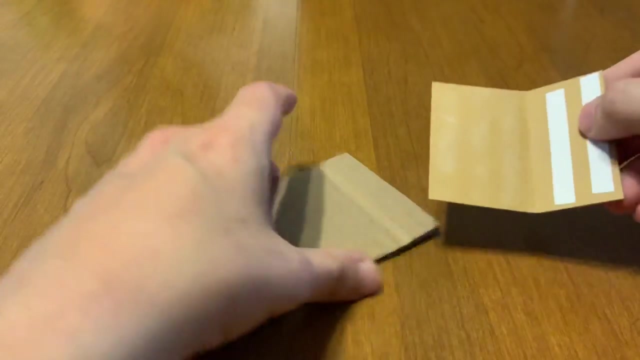 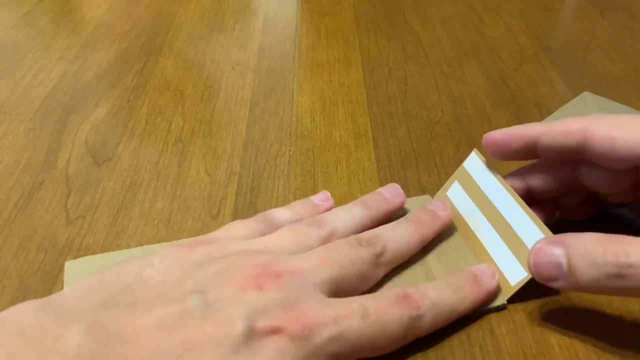 creates an edge of the- excuse me, the insert. I'm gonna go ahead and peel the other side of the tape So you can see there's the tape right there, Just careful not to lift it up. And with this I'm just gonna put it right on top. See how. 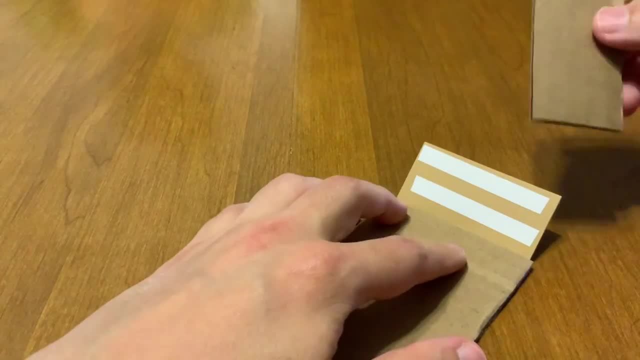 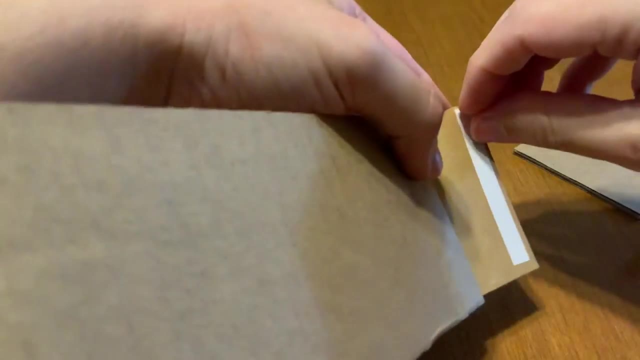 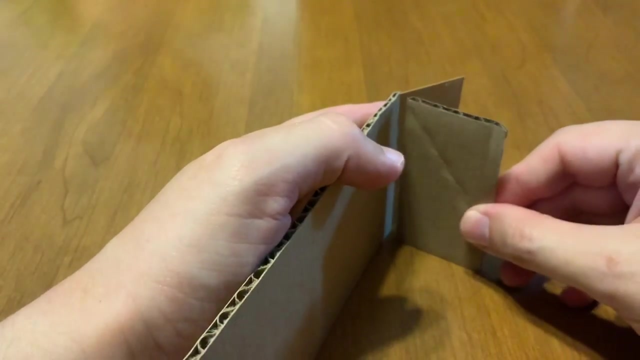 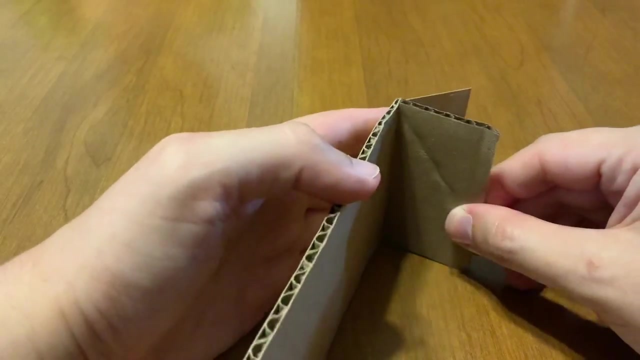 that fit. Okay, I'm gonna go ahead and peel the other side of the tape. I do one side at a time, Then this one what I do. I put it together the way that I'm gonna want it to be. Notice that how I have it. Okay, I don't have it. 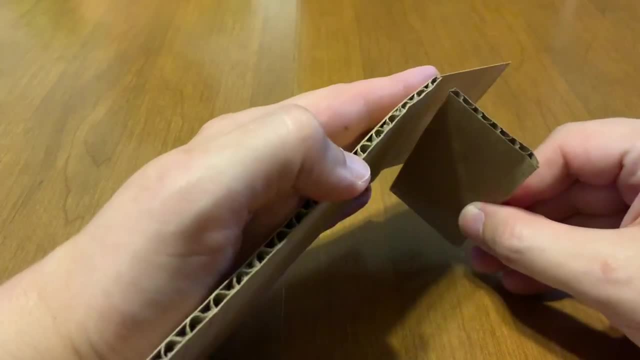 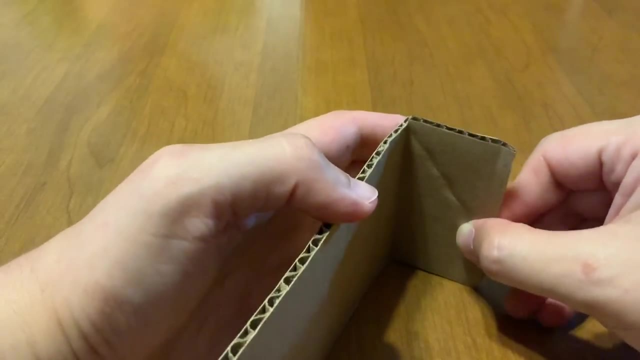 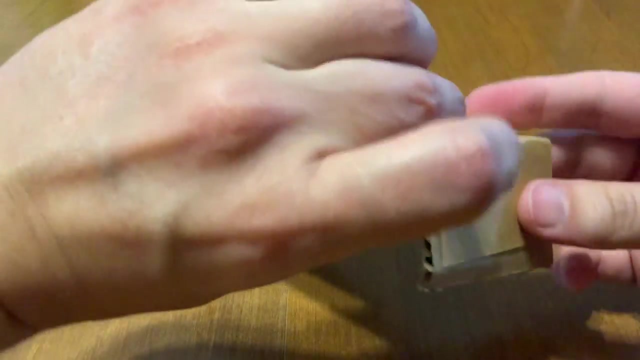 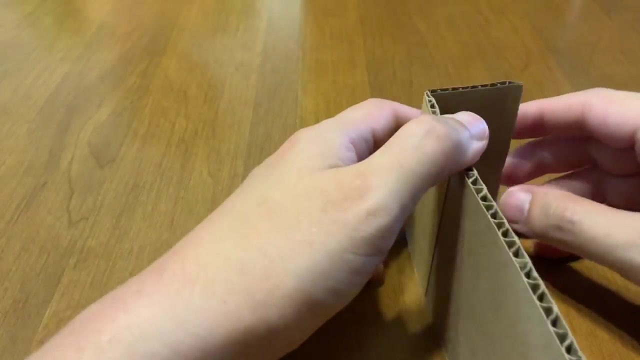 like this. I don't have it like this. I have it like this, Okay, not like this, Like that. I just make sure it's nice and flat And then I stick it together. So, as you could see, I have my first edge of my insert. Okay, I'm. 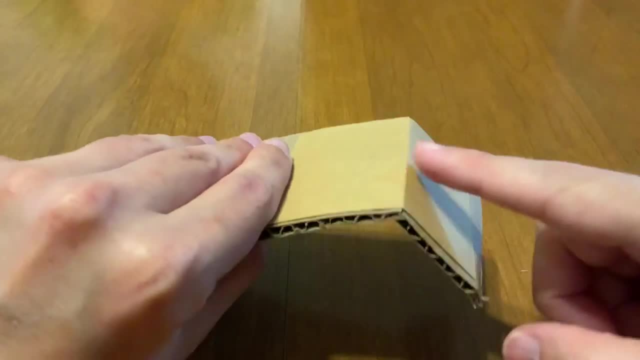 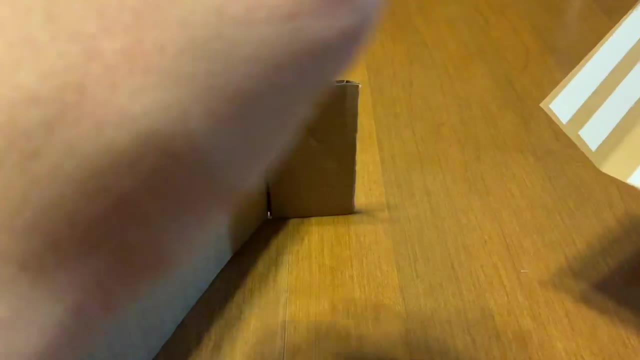 gonna go ahead and now, what I did on this, on what I did on this side, I'm gonna make sure that I could do it on this side, flatten like this so that I could fit the other one. I'm gonna go ahead and do the small side first, So I'm 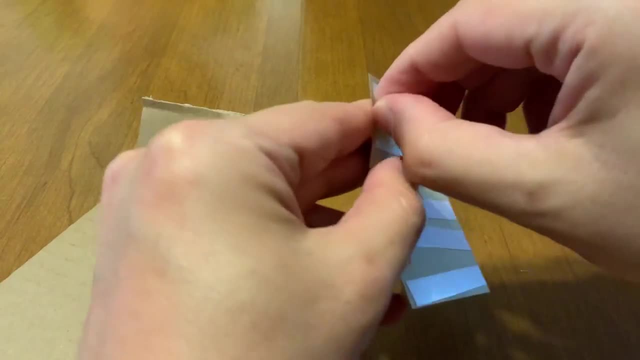 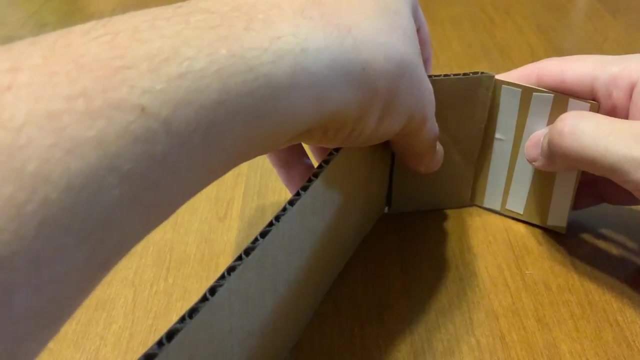 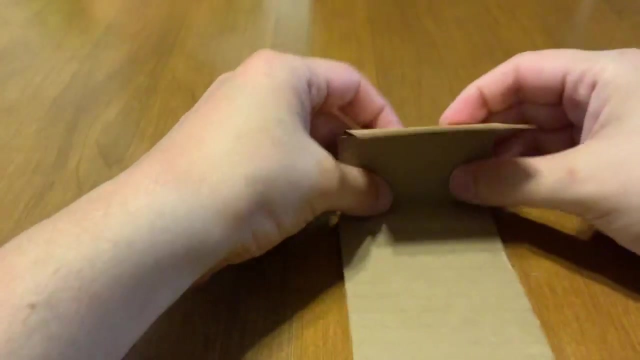 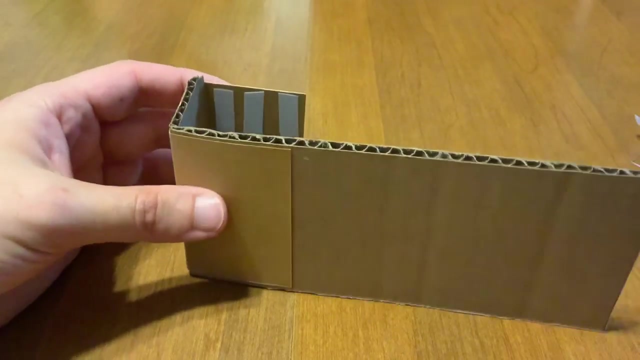 gonna peel The double-sided tape Once again… Taping it together. There you go. Now I'm ready to place the other side. You're starting to kind of see how it's starting to form, So I'm gonna go ahead and remove the others. 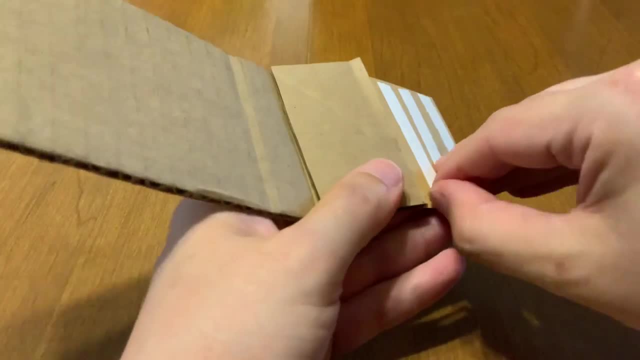 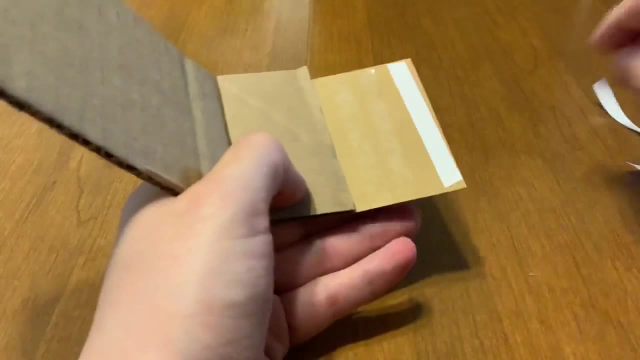 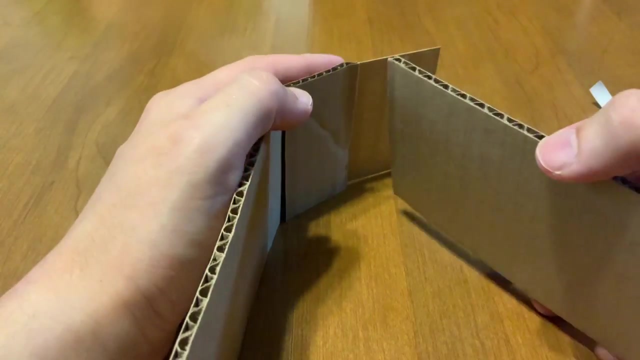 side like right here, it lifted up a little bit, no problem, I just go up on the other side, take it out the other way. always the solution to every problem. don't freak out, don't worry about it, doesn't have to be perfect, just has to work well enough. and once again, I don't want to put it: see how I can put on the. 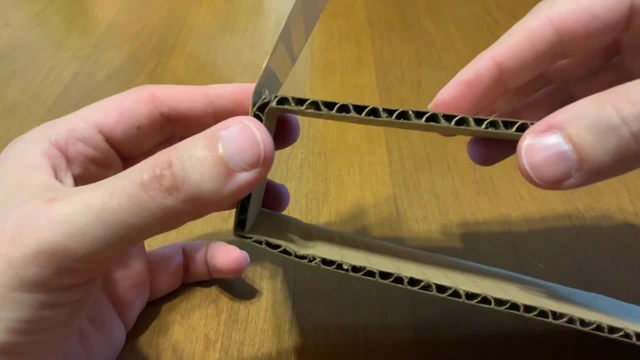 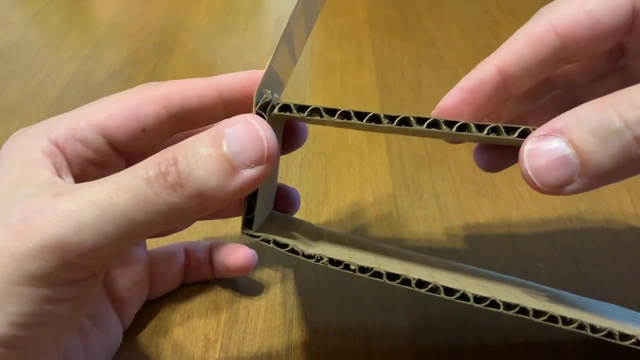 camera here so you guys can see it. I don't want to put it like this. I'm going to put it like this. okay, it just helps the integrity of the the insert. this makes it a weak insert. this makes a little bit more fun. I went ahead and did. 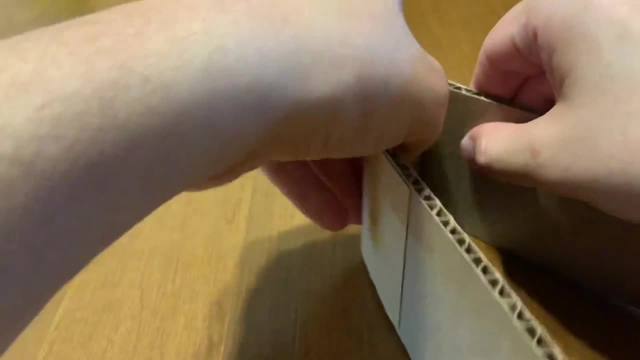 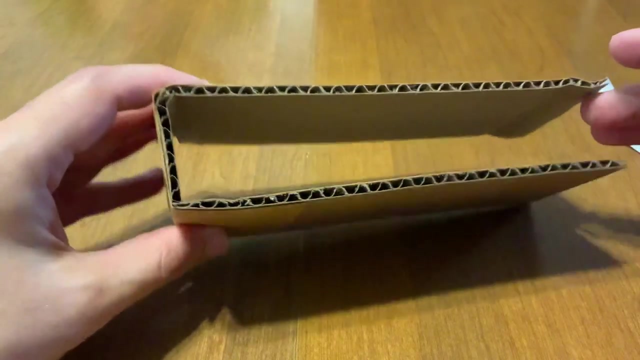 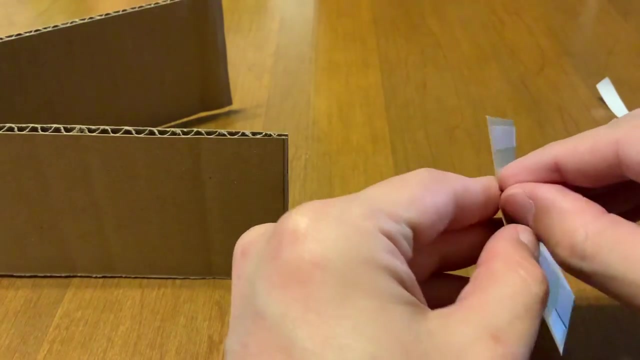 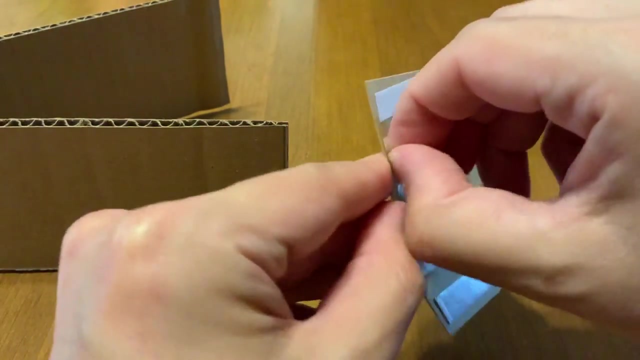 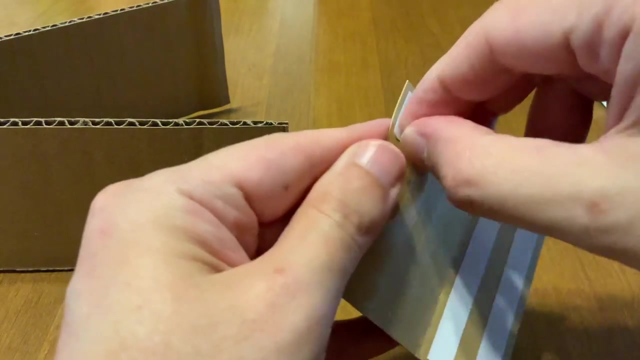 that, there you go, there's my insert, I already have it there and I'm just gonna go ahead and close this side once again. I'm gonna start with the bigger end this time. yeah, I'm already about to finish. uh, an insert right here and I. it took me barely just minutes, just minutes. 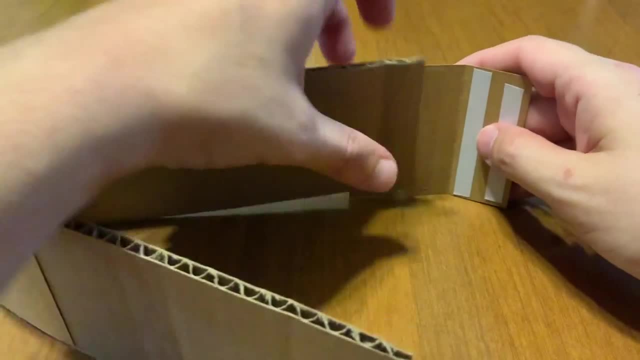 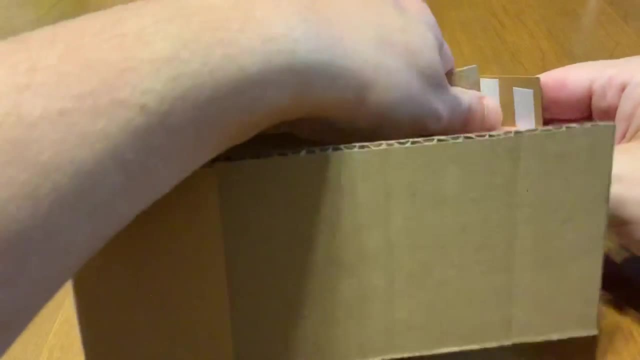 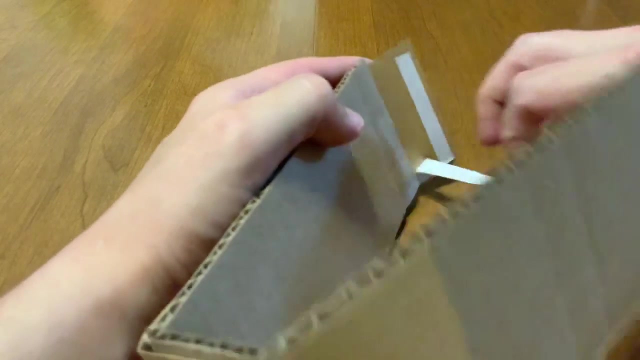 a lot of people think, hey, they think it might be. oh, it's going crazy here. it might be too difficult, too difficult to do this, it might be too time-consuming to do this, and just that thought my make it difficult, or me, make them not want to attempt it. but I assure you I 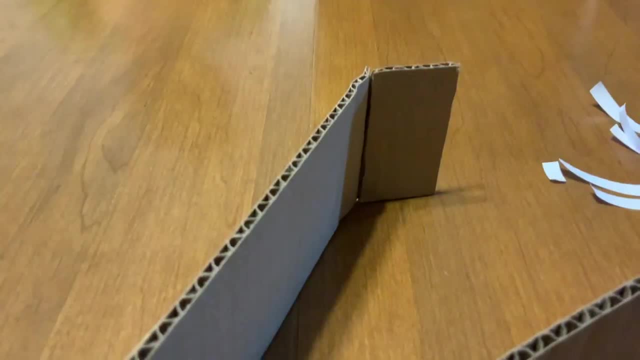 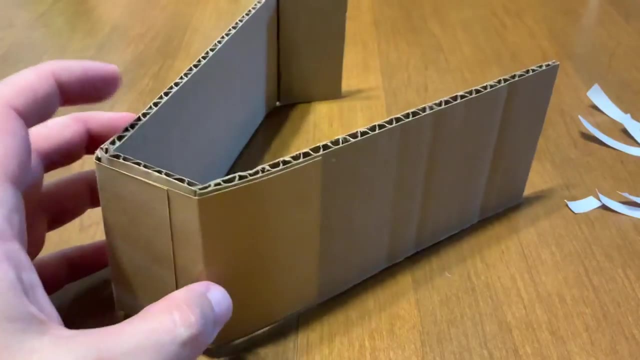 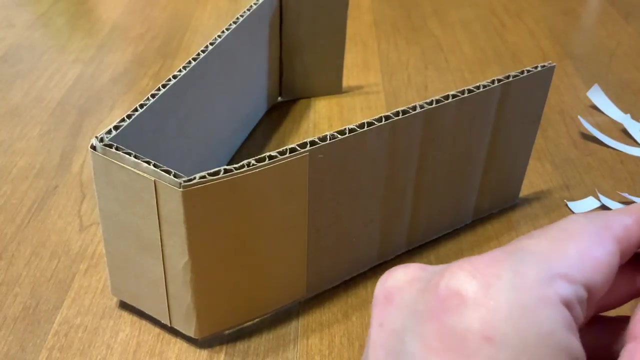 don't know why my camera's going crazy, I assure you, starting to see how it forms right. very good. I've done this so many times and it's made, especially when it comes to set up and tear down for my board games. it has been so, excuse me, so. 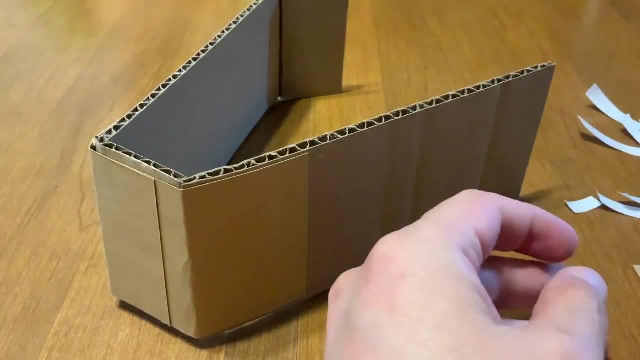 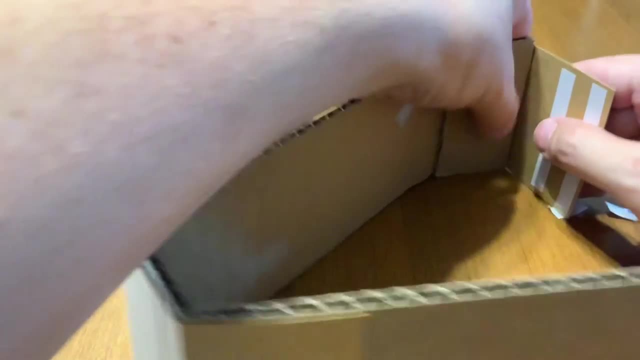 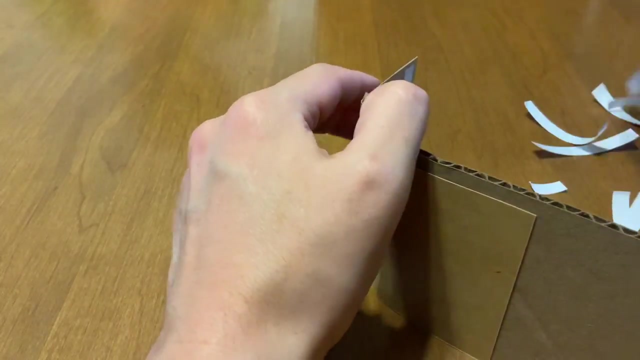 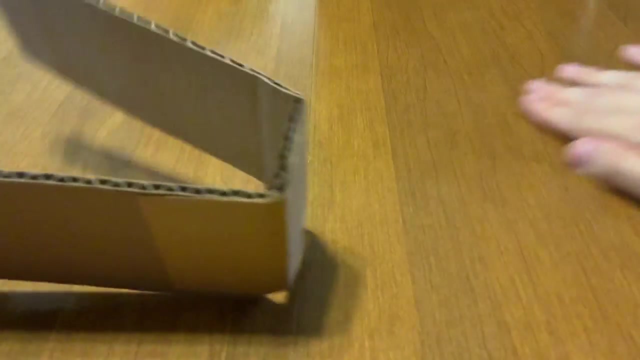 easy and enjoyable. it truly has- oh it truly has- made this set up of the board games that I have- and it's here down. so so good, simple, straight to the point- easy. I really have enjoyed it quite a lot. I'm just gonna go ahead and brush this to the side and finish it. 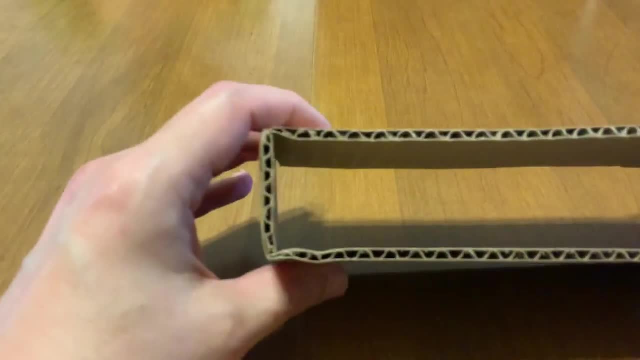 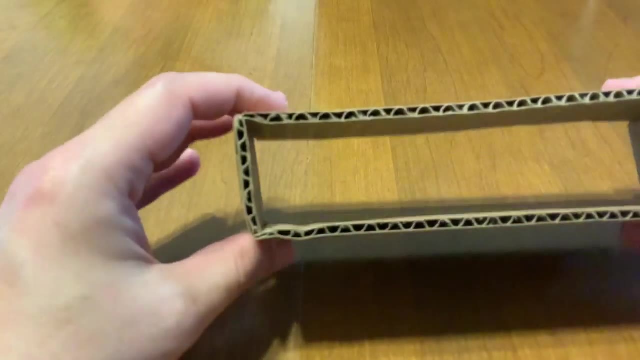 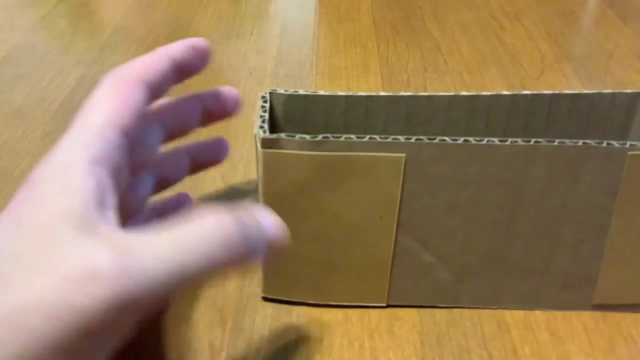 on to my next job. so basically, what I did to one side, I want to head and get it to the other side and, as you can see, here's my insert, so you could fit pretty much anything. notice that the dimension is very, very thin here. what this could be good for is, if you have those white cards, let me see if I could. 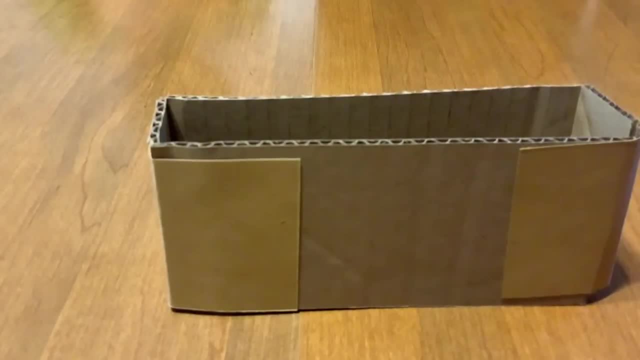 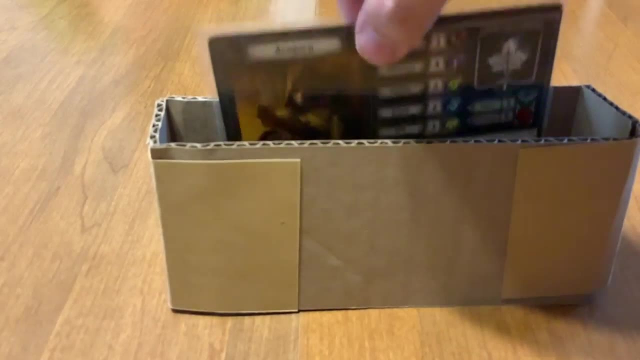 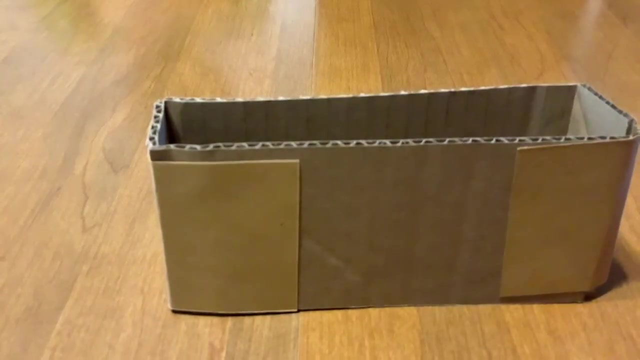 find one. I'm personally not going to use this for any particular game, I'm just doing it for an example. okay, this might be a little bit too big, but there you go. that's an example like one of these cards. I could have even made it a little smaller. 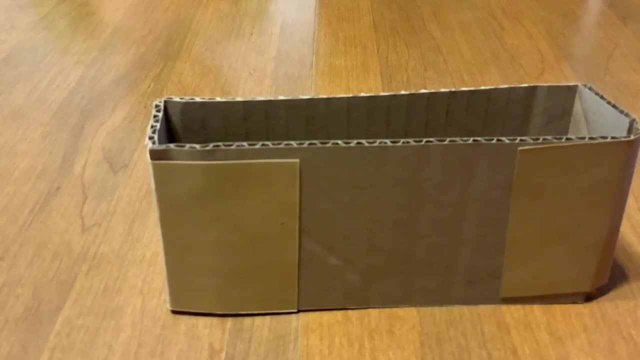 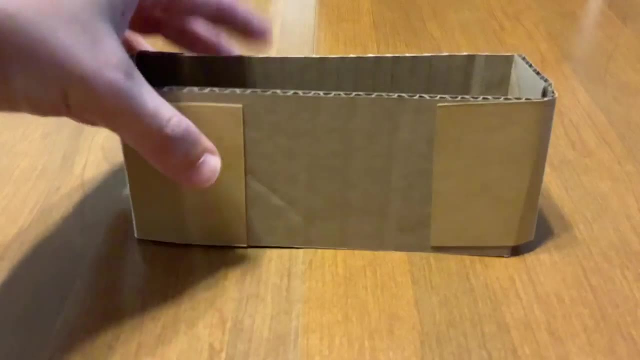 I'm gonna show you what my storage looks like for Journeys in Middle Earth, just so you can see. So, once again, this is how the insert would look and then basically what you do: you just fit it inside of the box. 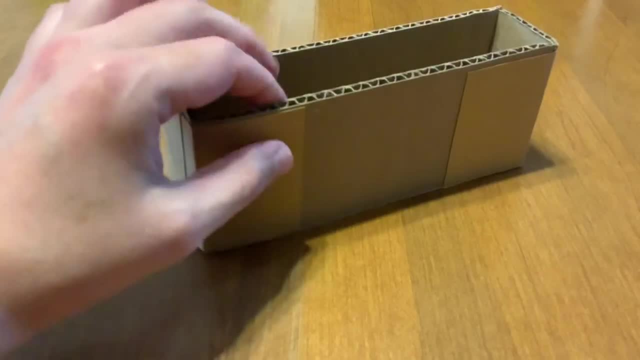 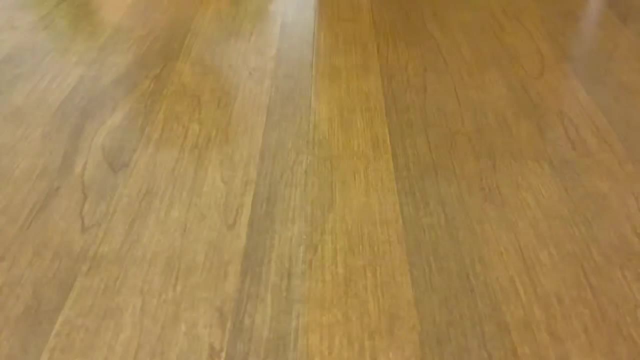 You fit it inside of the box. it's very sturdy, very reliable, it doesn't rip on you, it doesn't bend on you, it's so well made. Sometimes you make schemes so easy and enjoyable to deal with. So I'm gonna go ahead and 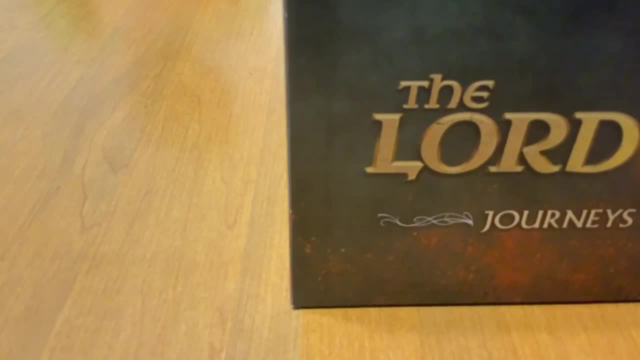 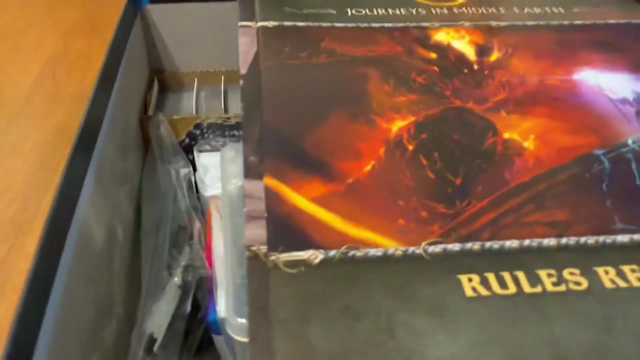 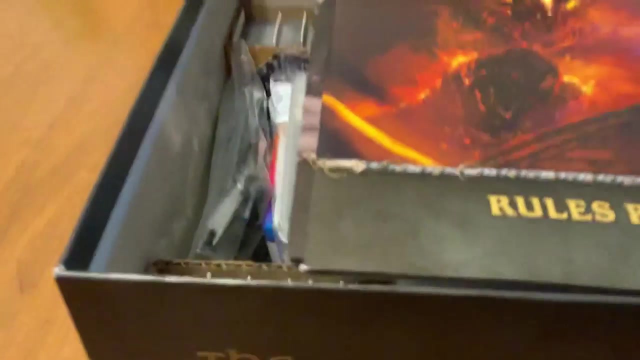 I'm gonna bring this in Hold on. All right, I just needed to lift this up, So this is my storage solution For Journeys in Middle Earth. this is how it looks on the top. I moved the box a little bit, but it looks like this. 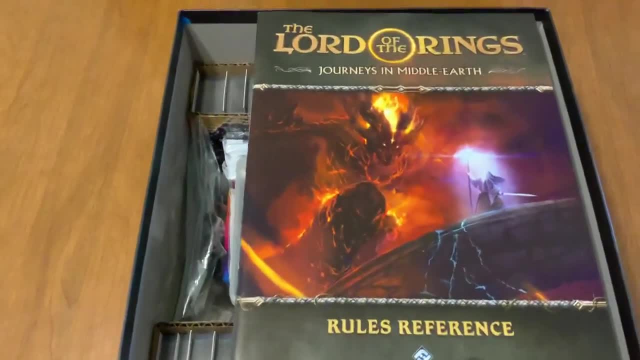 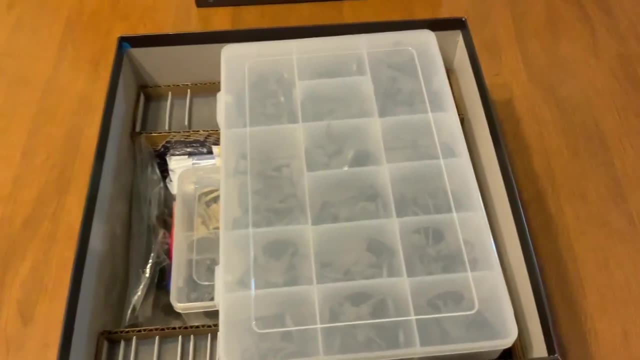 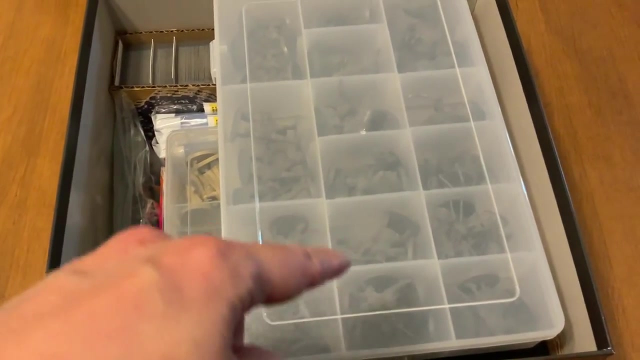 Okay, that's what it looks like on the top, So I'm gonna go ahead and remove the rule book and you'll see that right on top. I created an insert on the top and the insert on the bottom and I placed one of these cracked storage boxes. 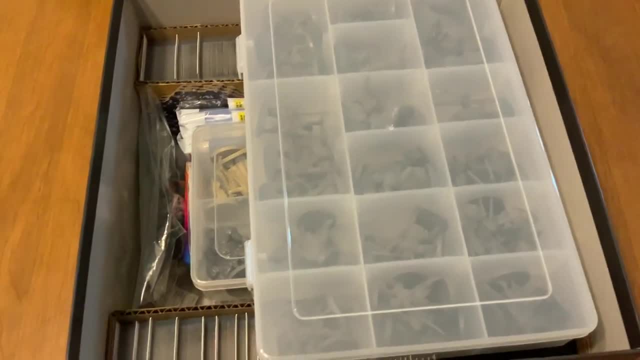 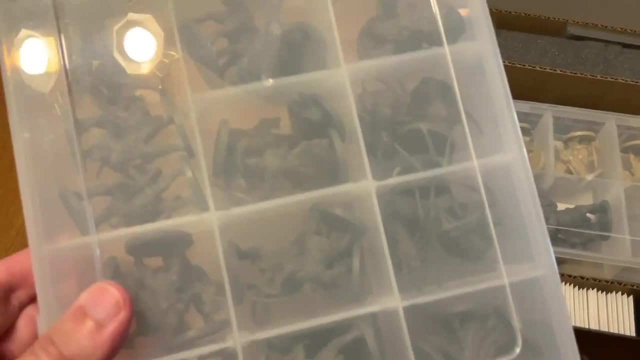 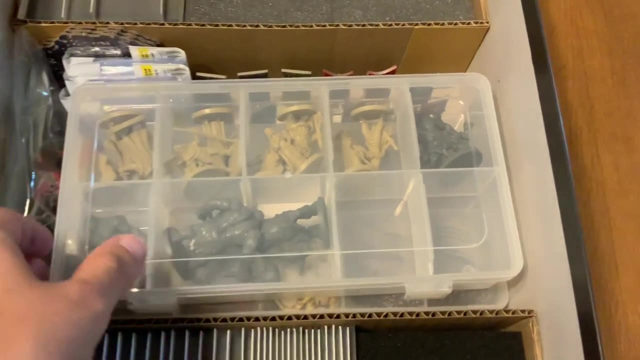 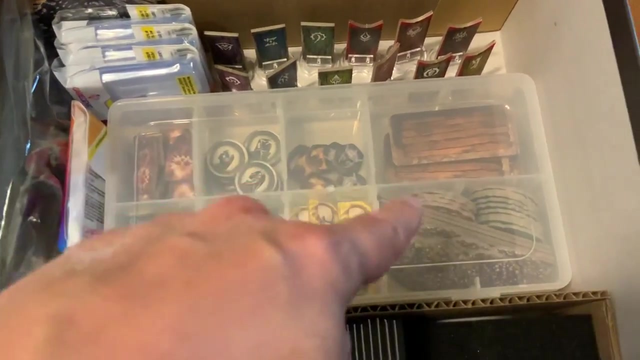 and this is where I put all my figures, my enemy figures, And right underneath that you'll see my heroes and the bigger enemies, and right below that, you'll see my tokens. Here are the tokens and here are the banners. 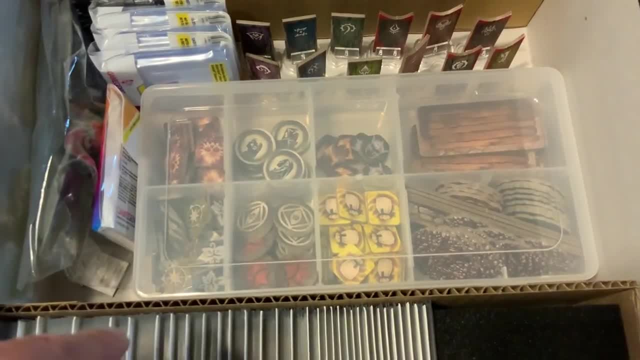 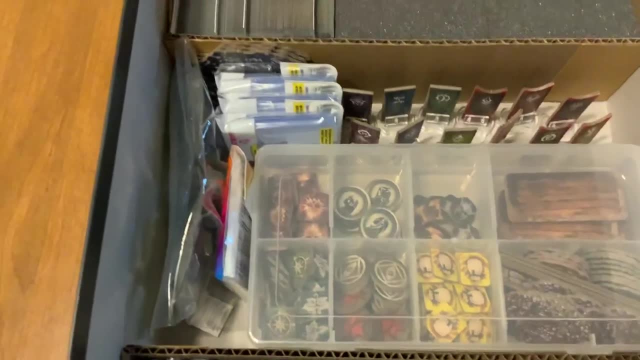 These cards right here are the sleeves I'm gonna use for the new expansion that I have pre-ordered and I'm waiting for it to come in October or November. and here's the big figure that I have there, And there's the insert. 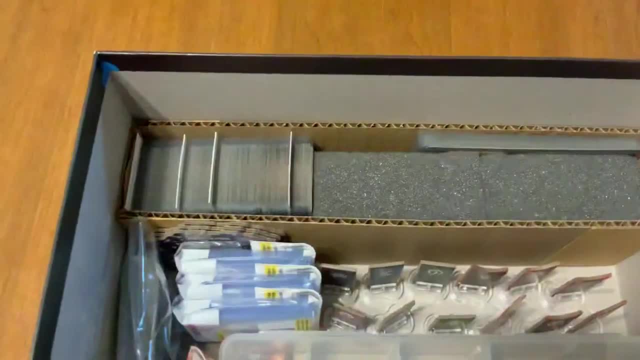 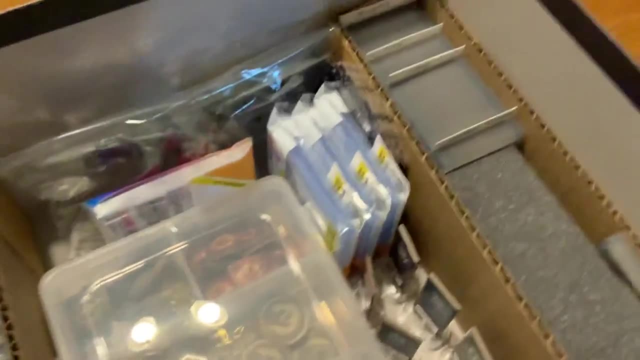 See, the same insert that I made. here is the same insert that I placed there and I have all of my. I created little dividers and let's see if you can read. there are my trinkets: titles, items. 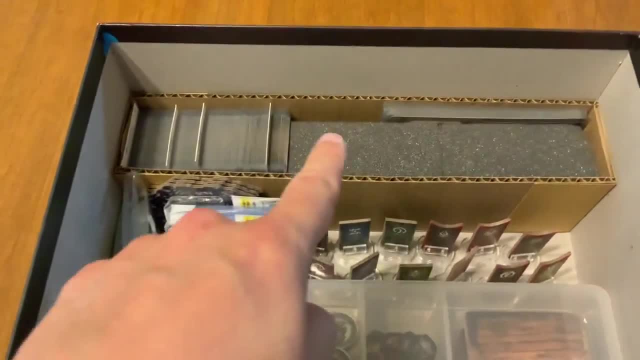 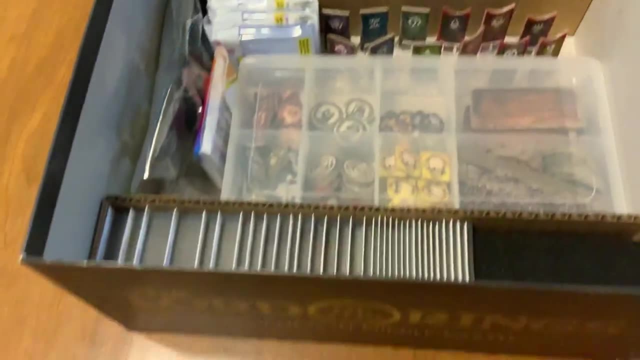 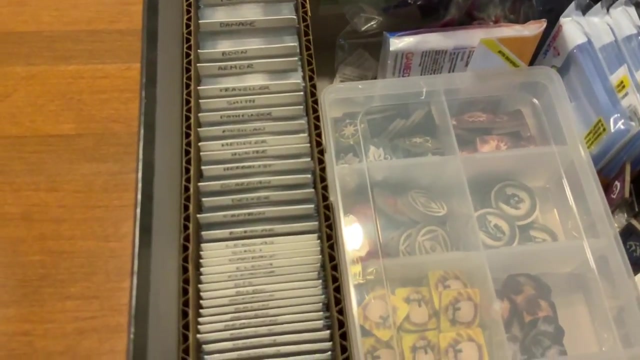 and my campaign progress. I put some of the card divider, the phone divider dividers right here and i ended up placing my character cards in between that space and on this edge. i did the same thing, and here you'll be able to see all my other types of. 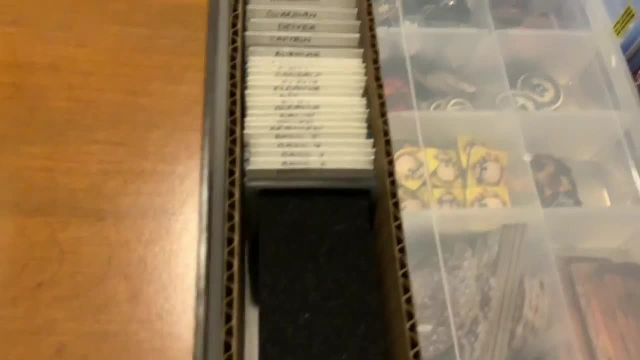 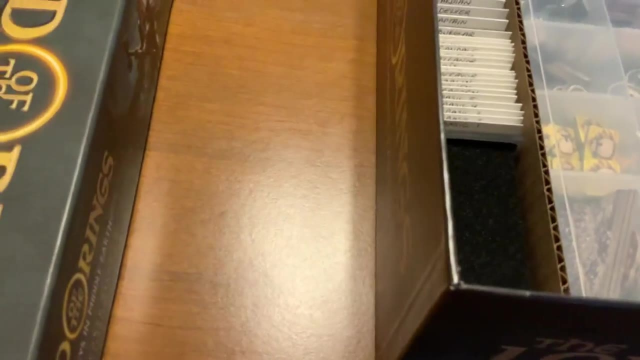 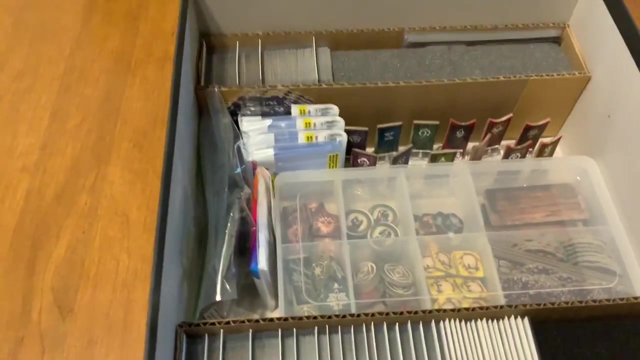 cards that exist. there are all the characters and i i placed different all the basic cards so up to five players can play at a time with me, which i always play solo, so it doesn't happen. so that's how i've stored uh journeys in middle earth. you might be asking: well, where are the tiles? 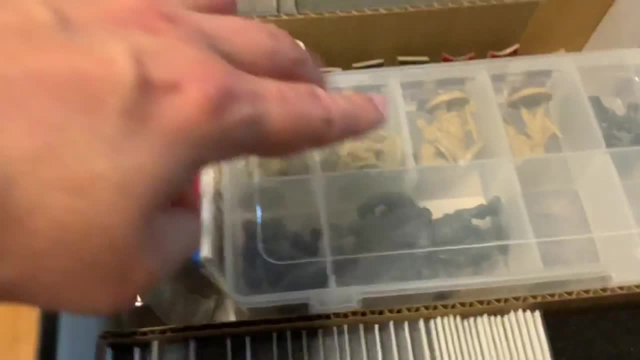 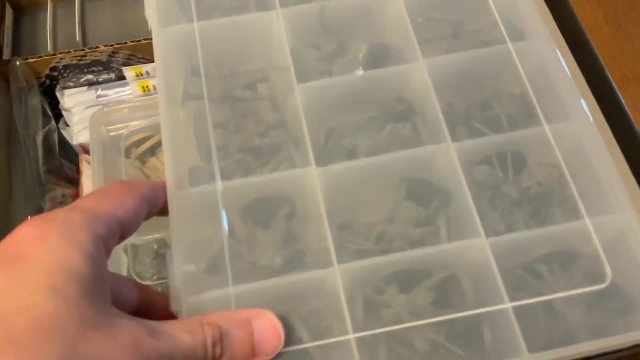 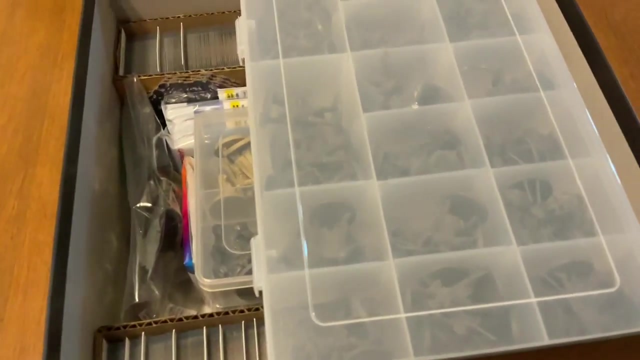 the tiles. i could have placed them here in the middle, but i ended up using the expansion shadows- shadow path- i think it's called the, but the expansion to this game is where all the tiles are being held. i i use that instead and it works. it works really well because i put it in alpha. 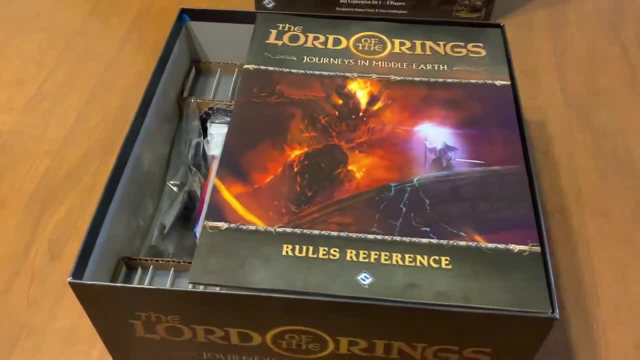 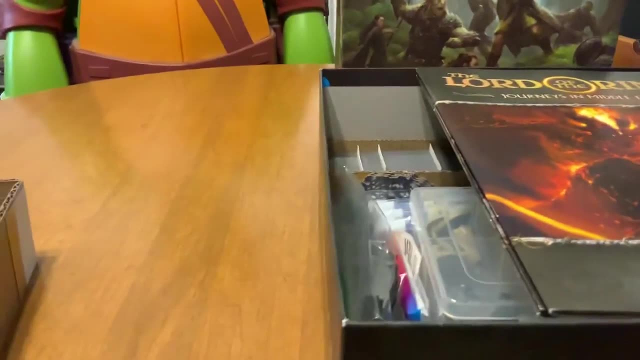 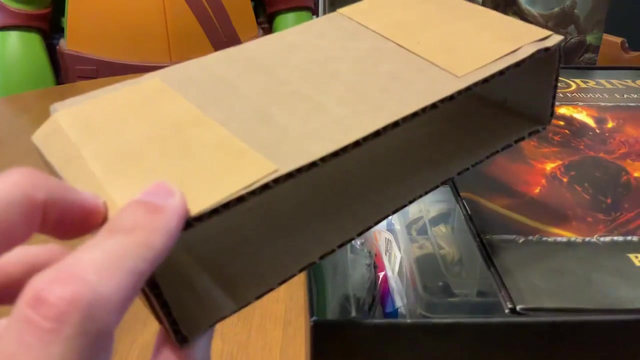 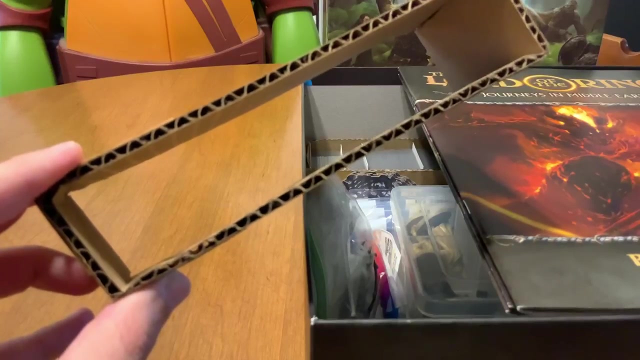 in a numerical order, so there very easy to read. so i just bust the game out and i just pretty much set up and take down this game very easily and it's all thanks to these little inserts that i created and i showed you. i hope this helps. i hope you're able to try it yourself and, if it, if it worked, let me know how it went. 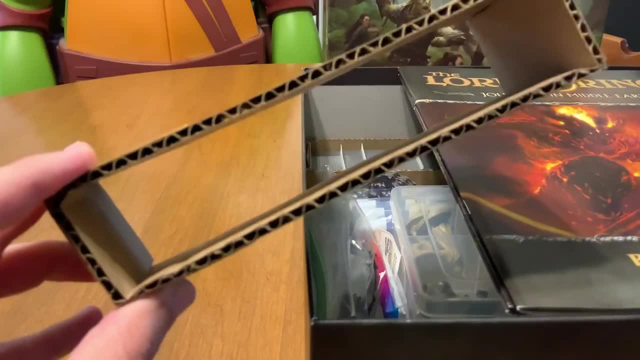 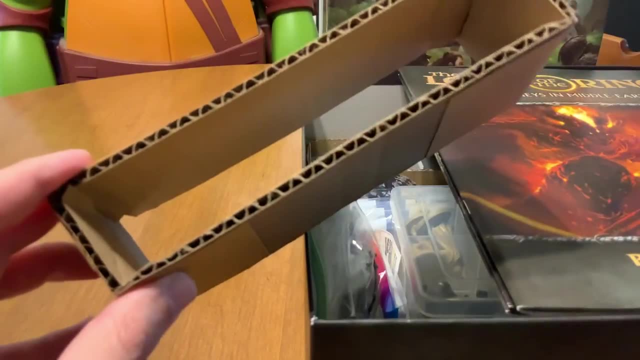 which game you used it for. i'm gonna do the next one for mansions of madness, second edition. i thankfully didn't need to do it for descent legends of the dark because in my opinion, the legends of the dark did a great job with the storage solution. i was able to use that box itself. 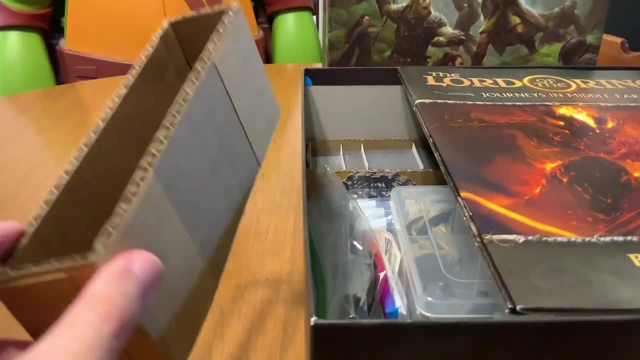 so just let me know if it helped you. this has been solo board gaming nights and i hope you guys have a great game night. take care.